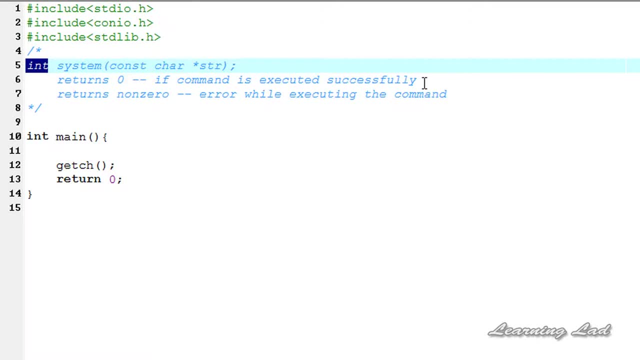 But typically zero is returned if the command was executed successfully. Else, a non-zero value is returned, which indicates the error. Okay, now we are going to see how we can use this function in our program. So, just for the demonstration purpose, what we are going to do is: 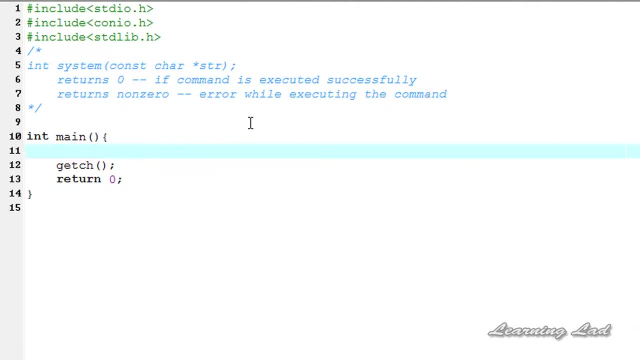 first we are going to check whether the system or the operating system supports the command processor. That's why I am going to use the system function inside the- if It's going to be- if- system of null, So if the command processor is not present in the system function. 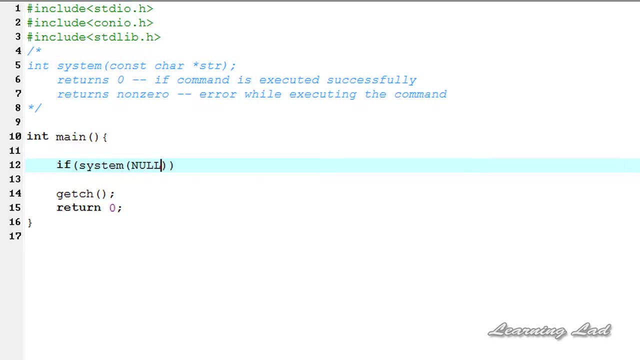 then it's going to return a value of zero. Else, it's going to return a non-zero value. So we are going to check that. if it is not equal to zero, then it's going to mean that the command processor is present. 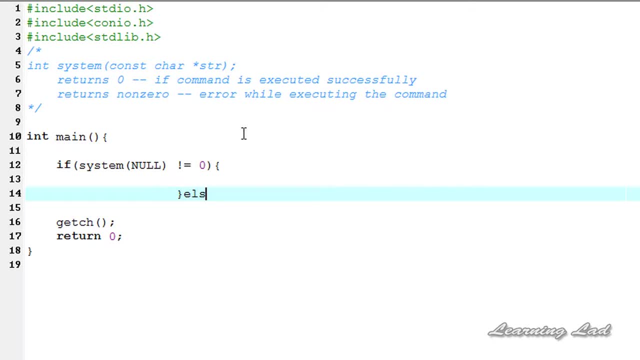 Then we are going to execute the commands there. Else we are going to print out the message saying that the command processor is not present. So I am going to use the foot test function And I am going to say: command processor is not present in your OS. 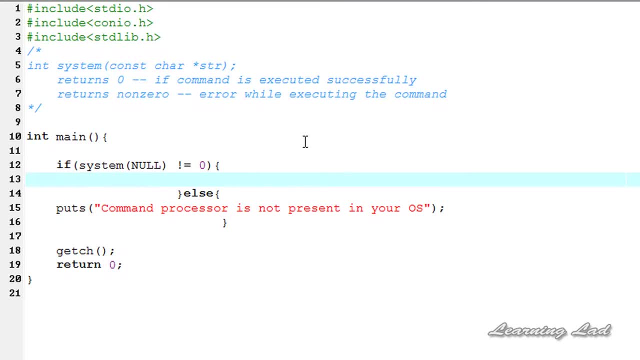 Okay, now here, if the command processor is present in the system, then we are going to use this system function to execute the commands. So it's going to be system and, as a parameter, we are going to pass the command. 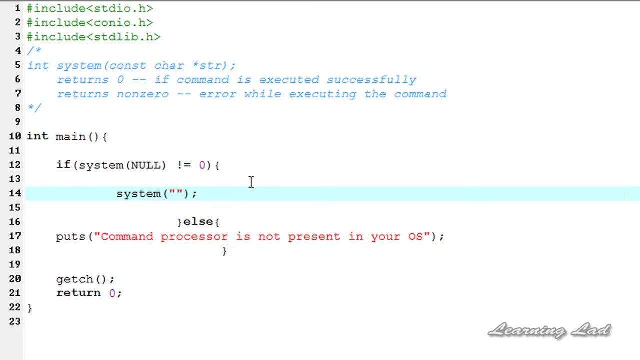 So in this case, for the demonstration purpose, I am going to pass the dir command, which is used to list the files and directories present in the current working directory. So I am going to save this one: Execute, compile and run. 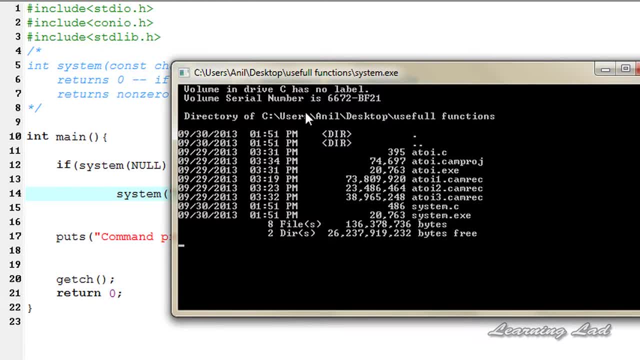 So you can see here the output of this dir command is listed. It just lists the files and folders present in the current working folder, which is, you know, causers anil desktop useful functions, And these are the files present in that folder.